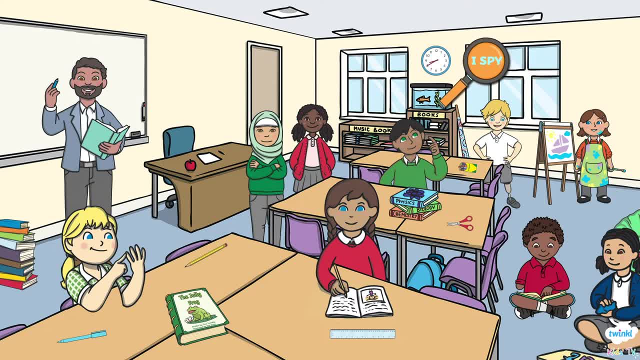 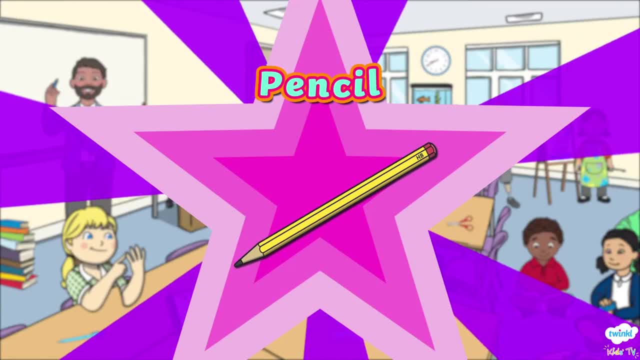 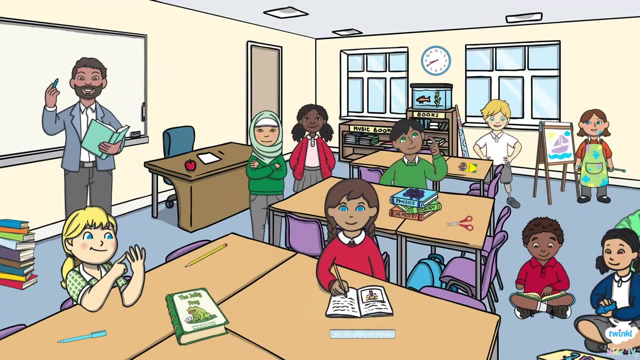 Can you see it? What could it be? You've got it: It's a pencil. Pencils are important for doing our schoolwork and practising our writing. What's up next? iSpy with my little eye Something the teacher might write in. 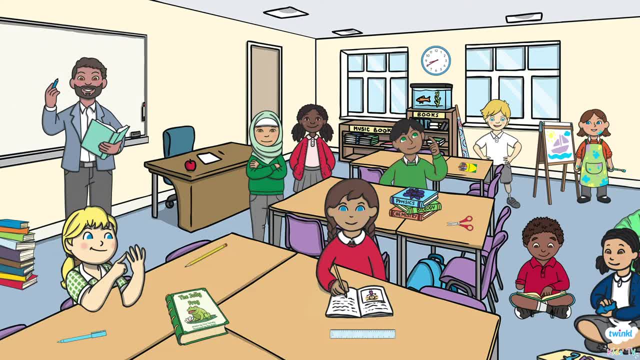 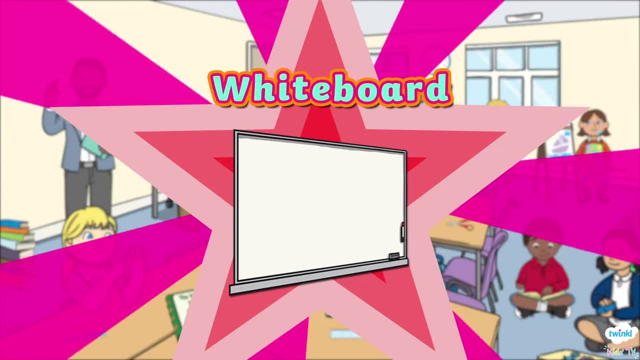 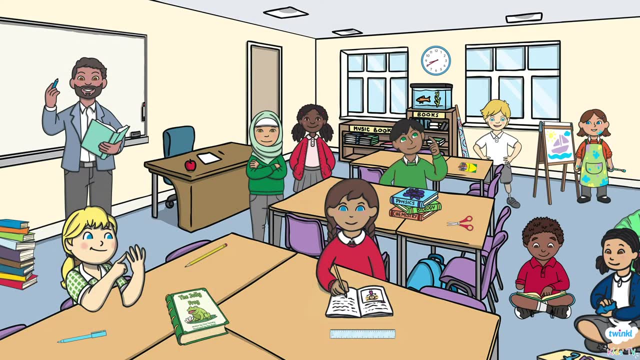 Something the teacher might write on. Do you know what it is? Well done, It's a whiteboard. The whiteboard is at the front of the classroom, so everyone can see. Great job. Now it's time for another. iSpy with my little eye. 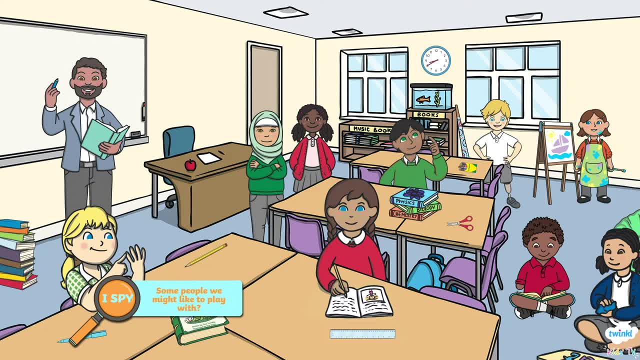 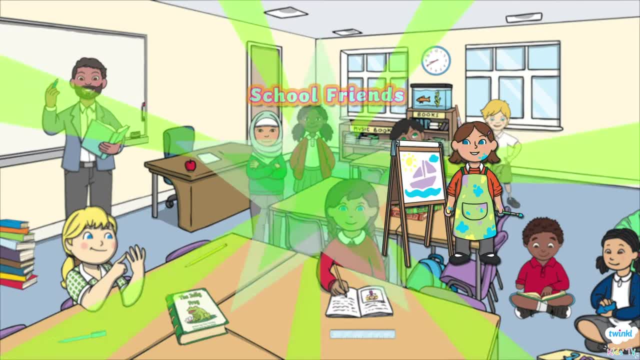 I spy some people we might like to play with. Can you see them? Can you see them? There they are, It's iSpy with my little eye. They're your friends. We can make lots of new friends to play with at school. 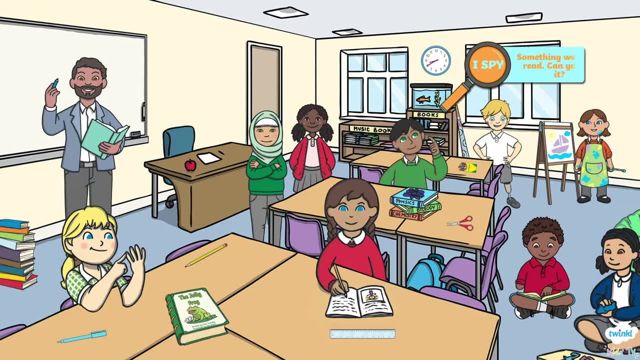 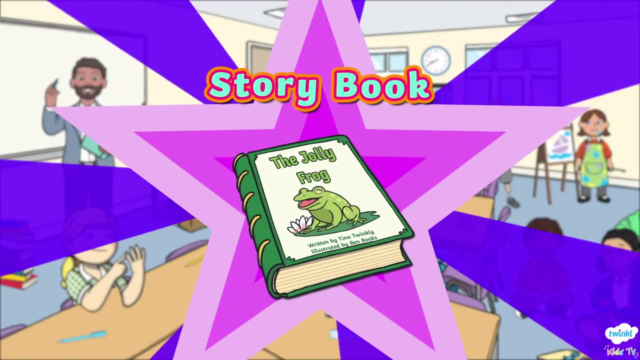 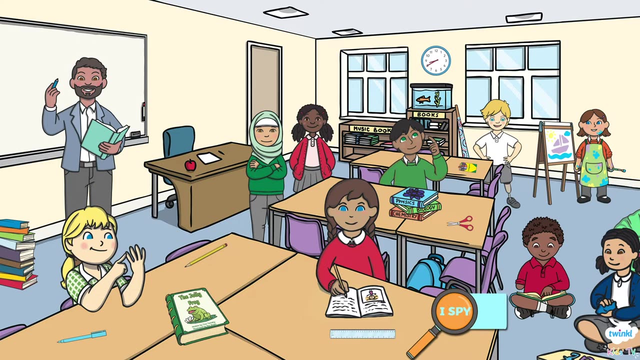 Now, what can we see? iSpy, with my little eye, Something we might read. Can you see it? You've got it. Well done, It's a storybook. We can practise our reading together at school. Next up, iSpy something we can use to colour or draw with. 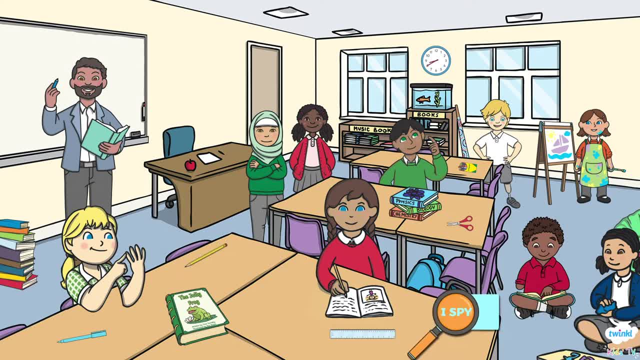 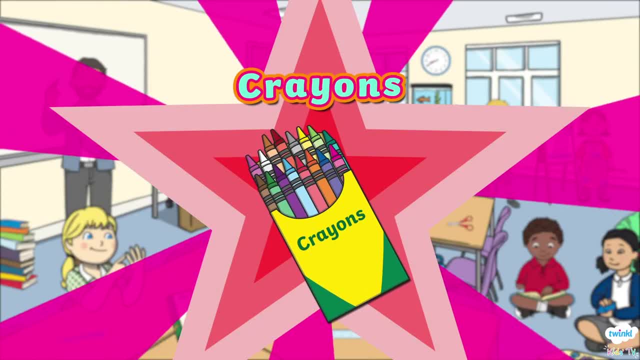 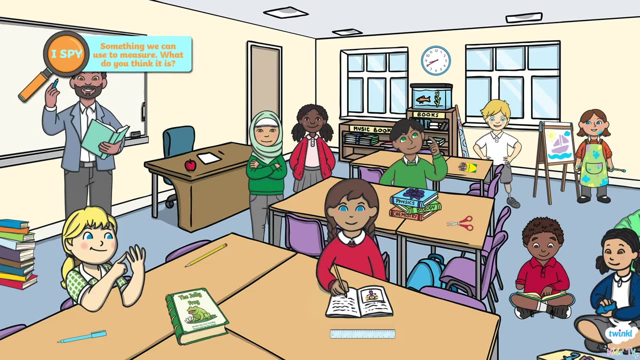 What do you see? Can you spot it There? It's crayons. We can use our crayons to draw some colourful artwork. What else do we have here? iSpy something we can use to measure. What do you think it is? 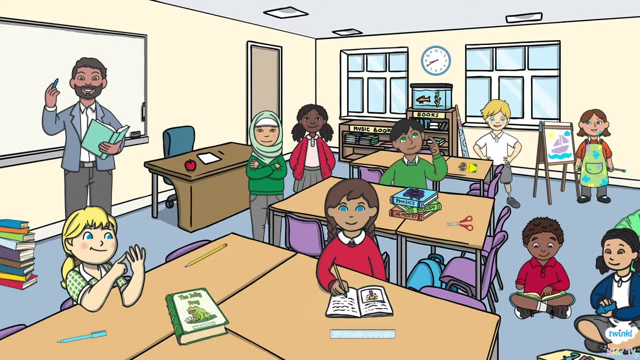 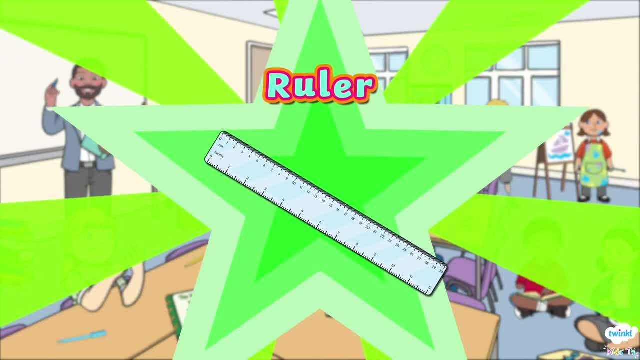 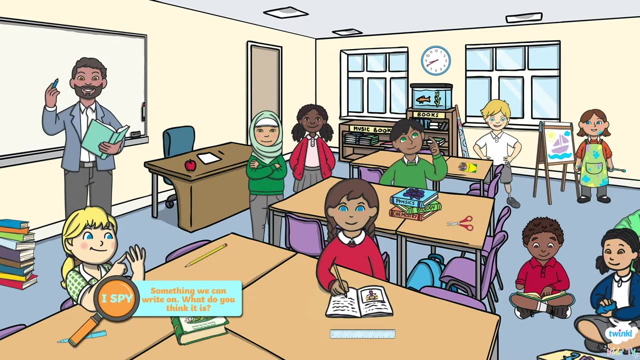 Can you see it? Can you see it? There you go. It's a ruler. We can use these to measure or help us draw straight lines. Now for the next one. iSpy something we can write on. What do you think it is?